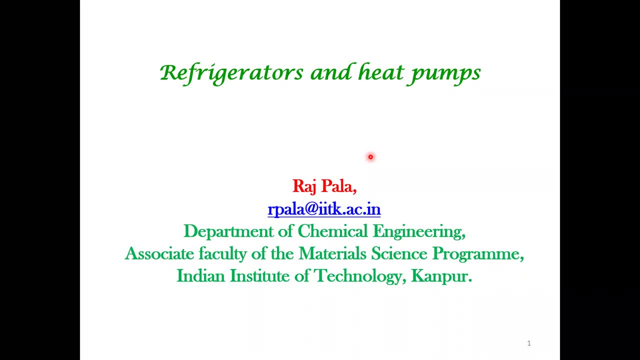 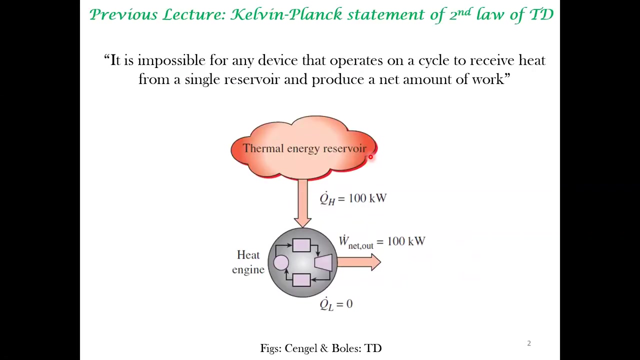 But what a refrigerator and heat pump does is it takes heat from a cold reservoir and dumps. it dumps some heat to the hot reservoir. So in effect, there is a transfer of heat from low temperature to high temperature. However, a work input is required to operate a refrigerator and a heat pump. So in the previous lecture we used heat engines to 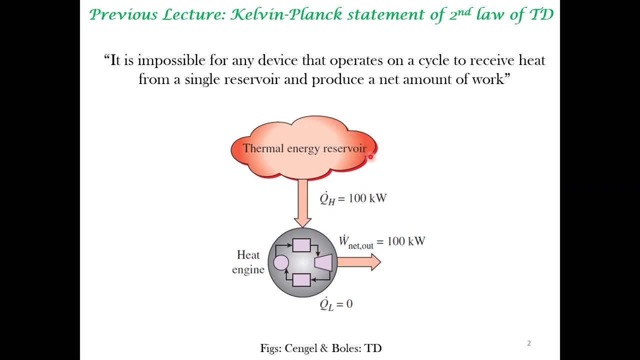 demonstrate a version of second law of thermodynamics, which is the Kelvin-Planck statement. It is impossible for any device that operates on a cycle to receive heat from a single reservoir and produce net work. In this case, all of heat is converted to work without any rejection of heat to the cold reservoir. Please note this is a negative statement. 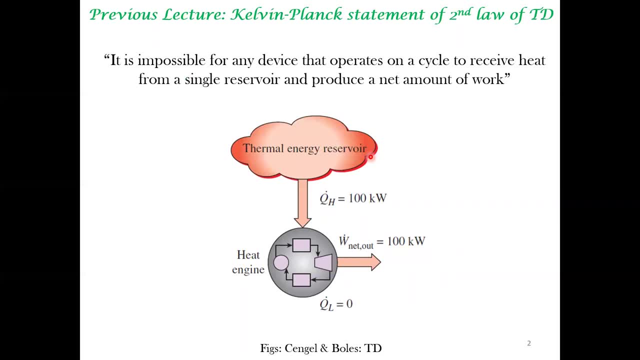 I mean in the sense that we are not proving something, we are just proving that it is impossible. So there is no way to prove a negative statement. The only proof, so to speak, is that there is no experiment that has disproved this negative statement. So all these negative statements, 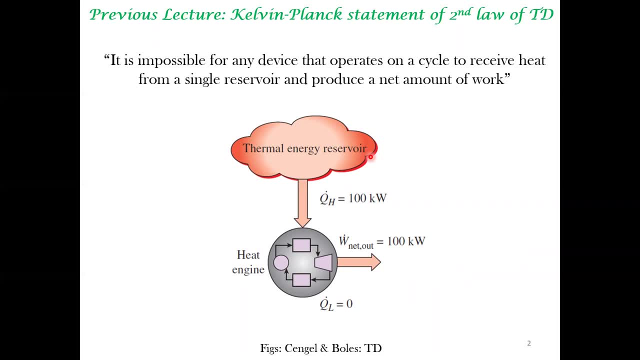 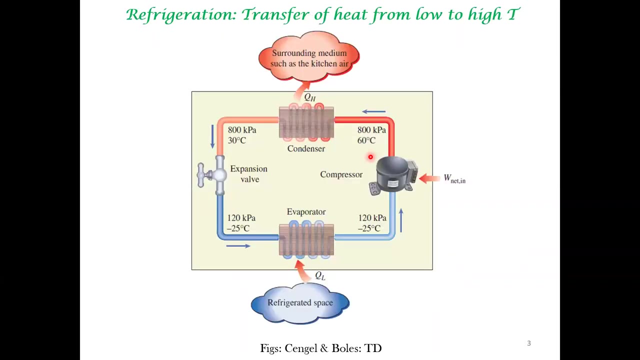 are proved, in a sense, that there's been no experiment which has contradicted this negative statement. So that's the way to think about these negative statements. So here this refrigerator is being explained. so what does the refrigerator contain? okay, so it contains a fluid again, like in the heat engine. 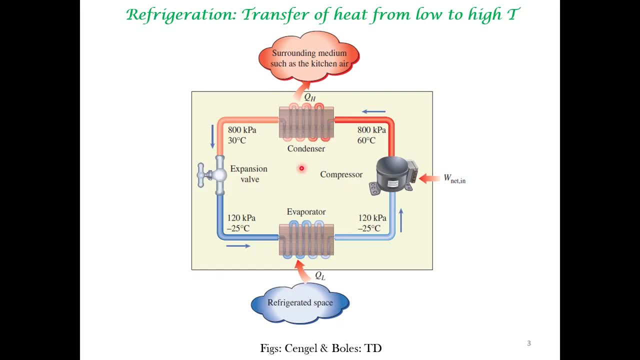 it's a fluid that goes around, so typically in this case, let's say, you have ammonia as a refrigerant. there are important refrigerant. ammonia was one of the refrigerant that there have been other successful refrigerant fluids that have been used in a refrigerator. so it's a cyclical process. it operates in a cyclical manner. 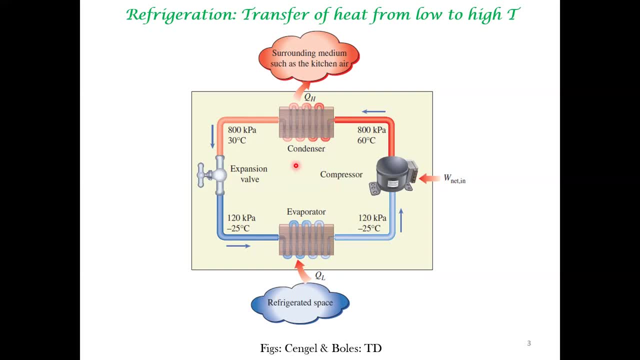 Let's see what we want to do. okay, so supposing you put some material which is at your room temperature into a freezer section of your refrigerator, refrigerator, so the heat from that material, let's say food item, which is at a room temperature, is supplied to a fluid which evaporates. okay, when something evaporates. 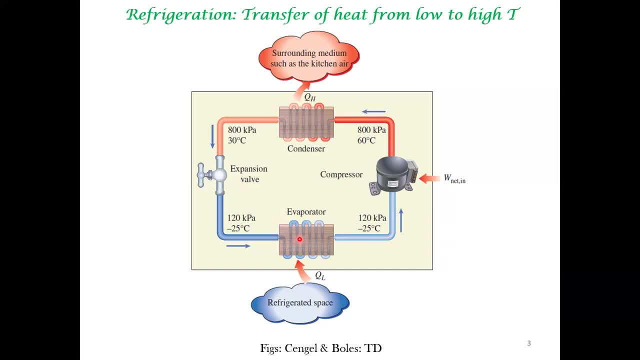 chemical bonds between the molecules are broken, so the heat supply goes towards breaking those chemical bonds and it evaporates the molecule. and then you are: these evaporated molecules are sent into a compressor. okay, so there is. this is the work input device. okay, so there is, work is put into a compressor. okay, so there is, work is put into a. 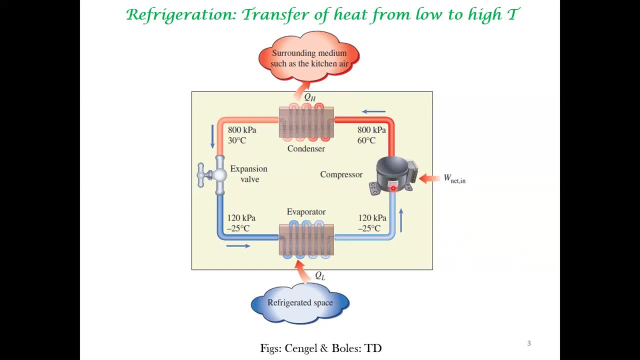 system. okay, you compress the material- these can evaporated gas molecules- you increase the pressure. not only increase the pressure because of the work input, the temperature also increases. so the fluid goes into this condenser section. okay, so this condensing section is what is, for example, a normal 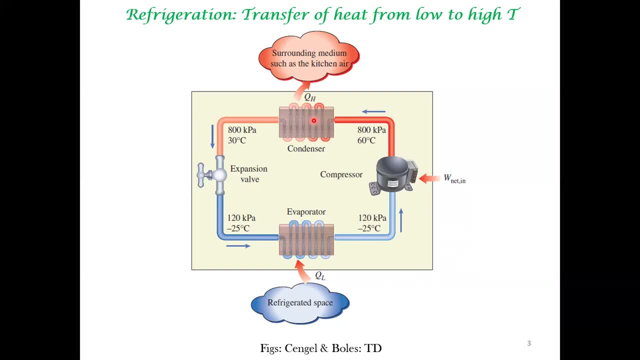 refrigerator. this is a set of coils that are outside the refrigerator, okay, so if you uh place your hand in this section, you can feel it is very hot, okay, so, um, all right, so, uh, so heat is rejected out of uh the coils, okay, in the in this condenser section, typically, that is. 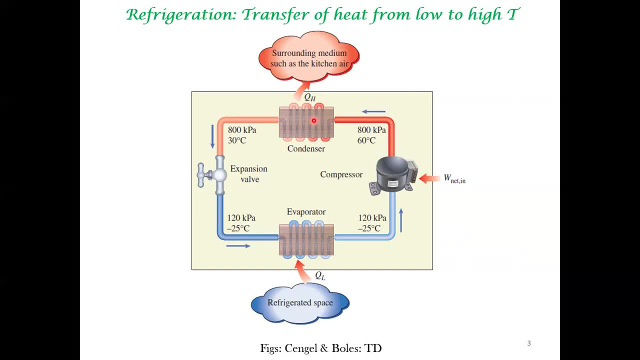 area which is hot. okay, so, typically, if you place your hand uh, you can feel uh that it is much warm compared to the rest of the refrigerator. okay, so heat is rejected uh, in a way, heat is transferred to the ambient atmosphere which is outside these uh condenser coils. 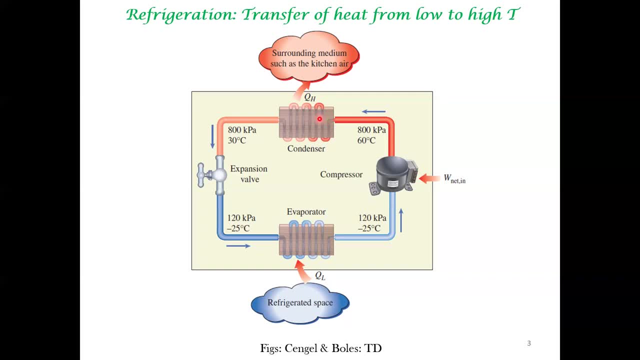 all right. so typically, why do we call something as a condense? okay, so condenser means typically gas. molecules are condensed into a liquid. again, new bonds are formed, uh, which gives rise to rejection of heat. okay, this is the opposite here, right, so here you supply heat, the more bonds between molecules are broken as it evaporates here. 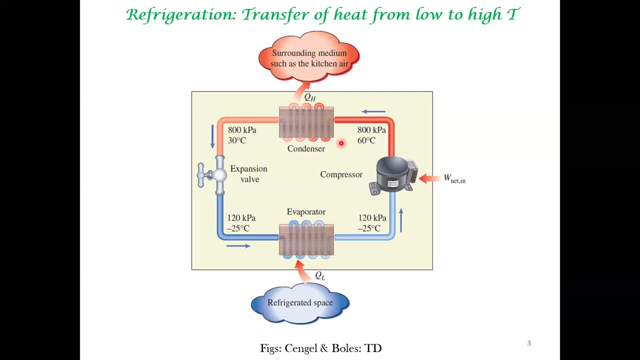 the new bonds are formed, uh, when gas molecules condense into a liquid which gives rise to generation of heat that is rejected via the coils of the contents. so here, because of the rejection of heat, temperature goes down. and then there is this is at a high uh pressure. 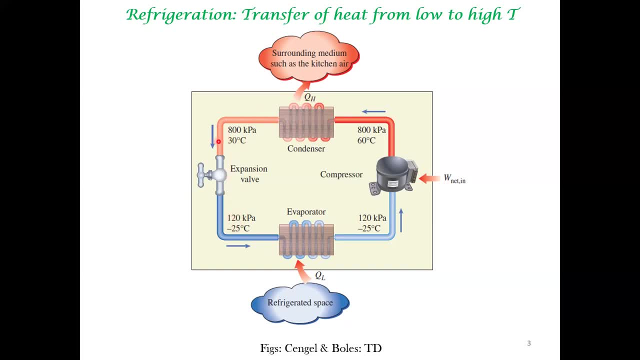 and this, as you can see, when this high pressure fluid goes through a certain kind of valve- okay, expansion, there are capillary valves, and so on- what happens? there is decrease in pressure and temperature. okay, so, and then the cycle continues. okay, so, this is this refrigerator operates through. 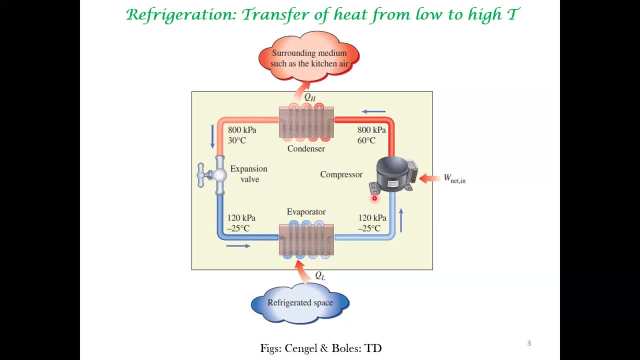 a vapor compression cycle. there are different uh engineering principle, different design uh approaches to uh a refrigerator. in this case, what we have demand elaborated is a vapor compression refrigerator. okay, so, uh. so this is exactly the opposite of heat engine. in what manner? uh, there is a similarity in the sense that both the heat engine and refrigerator are cyclical devices. 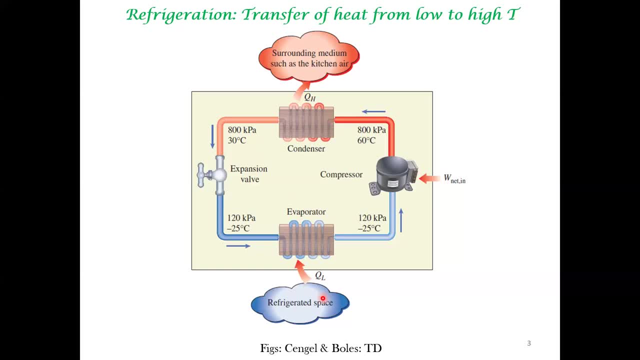 but a refrigerator. what it manages to do is take heat from a cold reservoir- okay, and then reject that heat to a hot reservoir- okay. so this is. and then there is some work, input into this cycle, right. so this in this way, this is heat engine run and reverse. all right so. 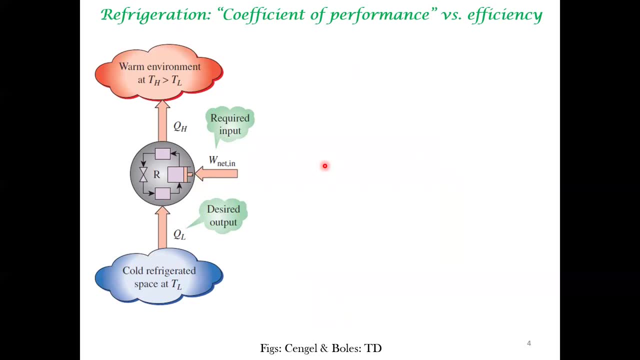 how do you think about an efficiency? okay, so there's a reason we don't use this word efficiency here. we will see why. so a way to think about the performance of a refrigerator is by computing the coefficient of performance. we'll define what that is. uh, so so what is that we want to achieve? we want to achieve heat removal from a cold reservoir. 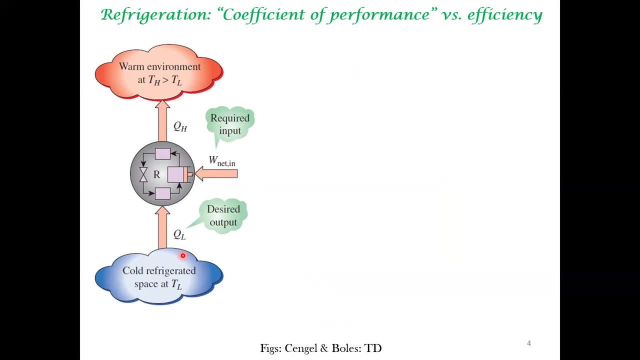 right. so that's what we want to be doing, right, we want to remove heat from a cold reservoir, and then, for accomplishing this, you supply some verb to a refrigerator that operates in a cycle. okay, so how do you think about this coefficient of performance you define like an efficiency. 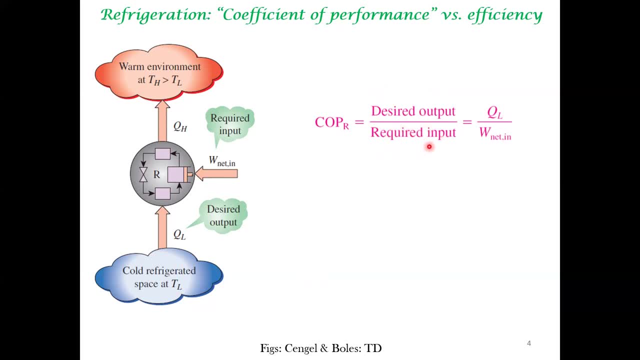 okay, this is what is desired and this is what this input into the uh device, right? so the desired output is heat that is removed from the cold resolution, right? and then what you have put into the system is the verb. okay, that's what is put into the system, because it operates. 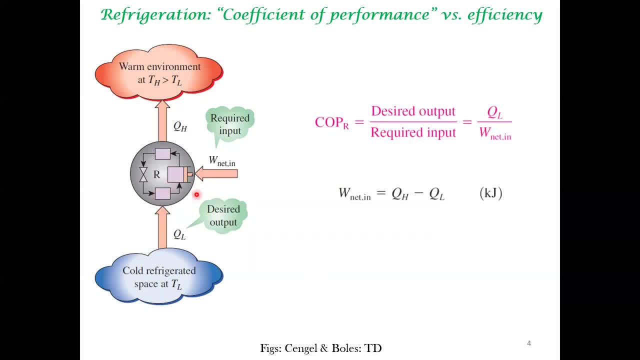 along a cycle. uh, by first law we can do this balance right. the net work in is because of a net heat transfer. substituting this into this formula, we get this quantity. so if you see this quantity, the coefficient of performance for a refrigerator can be greater than one. 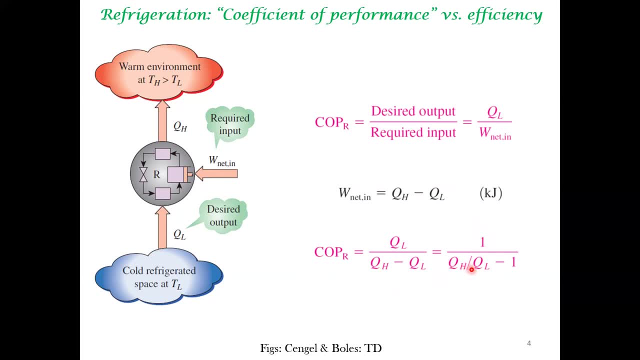 that is the reason why we don't use efficiency of a refrigerator, because efficiency, typically we say it's it's in between zero to one or zero to hundred percent. you don't see efficiency greater than 100% or greater than 1, right, So to avoid this weird number, efficiency being greater than 1. 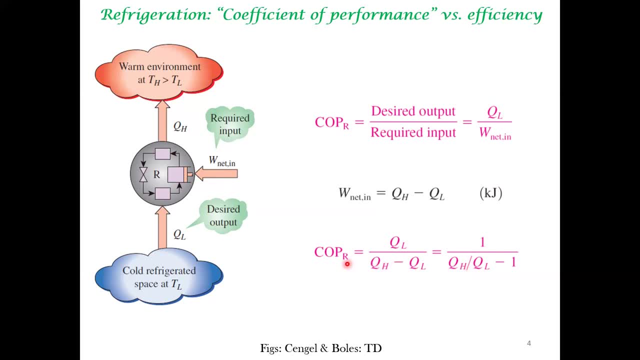 or greater than 100%. we use this. we call this quantity, which is like efficiency. okay, We call this quantity a coefficient of performance. right For your performance to be high, in this case, the refrigerator performance to be high. this should be low. 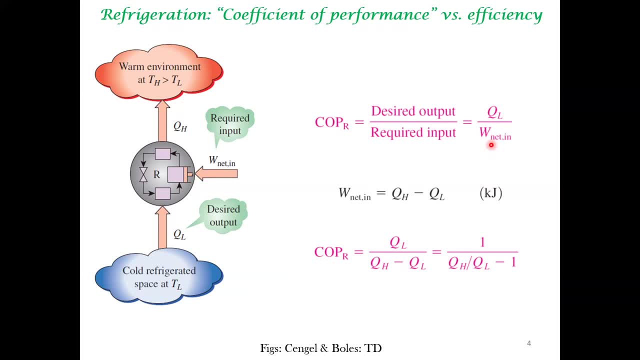 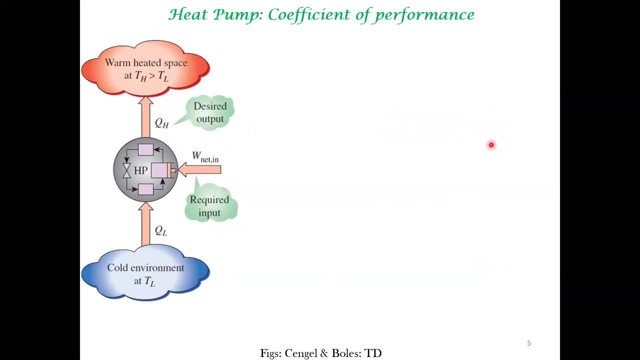 right. So in a sense it is like efficiency, but this can be greater than 1.. There is a related device called heat pump. okay, So this, if you look at it again, there is a transfer of heat from a cold reservoir to a hot reservoir. 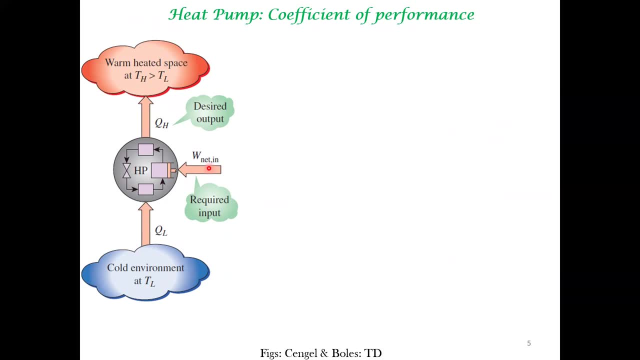 and work in it okay. So in what way this is different from refrigerator? The functionality of this device is different. In a refrigerator, the functionality is on removing heat from a cold reservoir, but a heat pump is used for keeping a hot reservoir warm. okay. 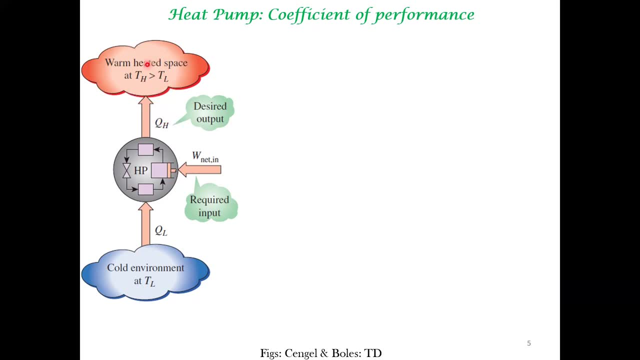 So you want to supply heat to this place so that this is kept warm, okay, So where do you use it? So typically, it is used in, let's say, winters in Western countries. So typically. so there is Atmosphere outside the house, okay. 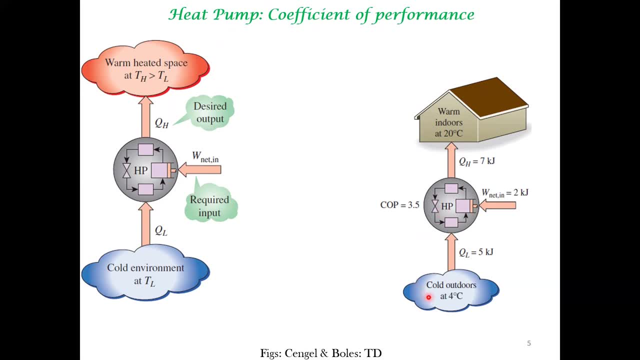 This is a residence. here, Atmosphere outside the house is quite cold. It's a four-degree setting, okay, So you take heat from that place and then you use it for keeping the indoor warm. The heat that is available is only from outdoor environment. 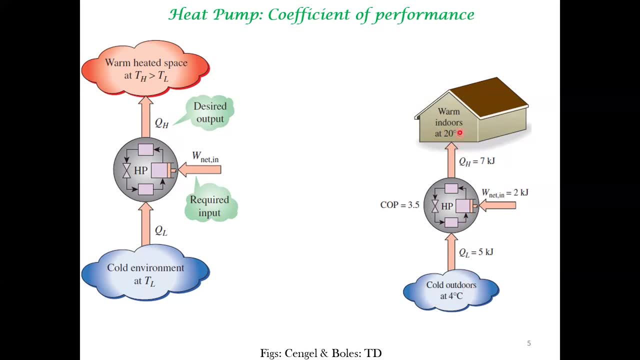 So you use that to keep the indoor of Inside your house? okay, So you want to keep it warm, okay. So, in effect, you are still transferring heat from a cold reservoir to a warm reservoir, The warm reservoir being the room where this device is operating. 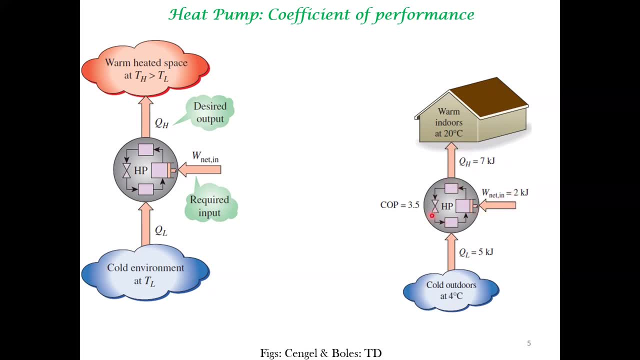 Okay, so again there's work, input, and this heat pump is operating in a cycle, effectively moving heat from a cold reservoir to a hot reservoir. Again, you can think about the coefficient of performance for a heat pump. How do you think about this? 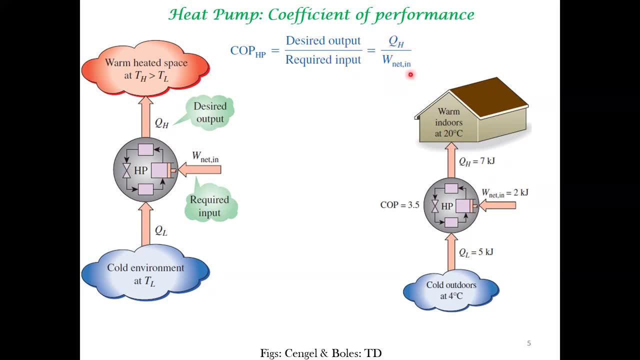 There is this desired output in the numerator and work input in the denominator. So for the coefficient of performance for heat pump to be large, this needs to be small. Putting this together, we can use the first law because it operates in a cycle. work network can be related to QL and QH.